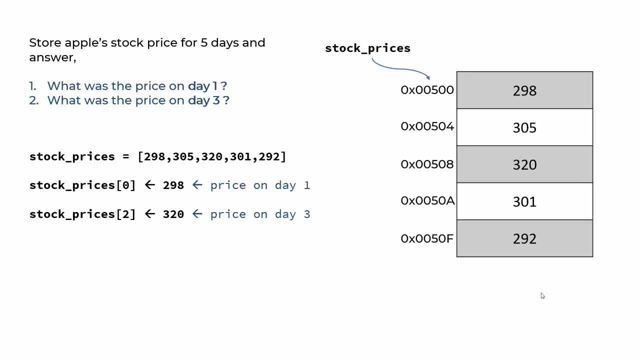 the variables In data stock prices in my Python program is a variable which it will store on these type of memory locations which have addresses. so this hexadecimal number are the addresses on RAM. Now, if you have the ability to open your computer and if you look at the RAM and let's say there is some way of 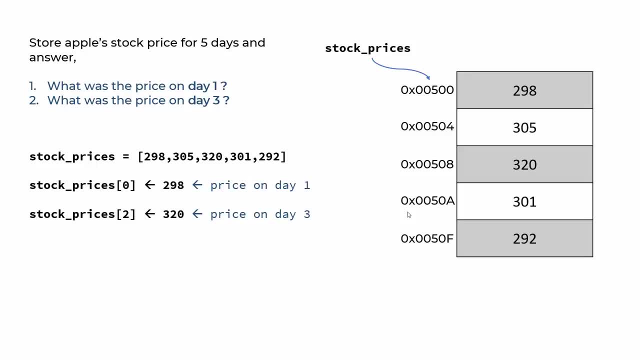 visualizing what is stored on that RAM. then you will not be able to see what is stored on that RAM, but you will be able to see what is stored on that RAM. Notice that the numbers are stored in bits, ones and zeros. So the diagram that I have. 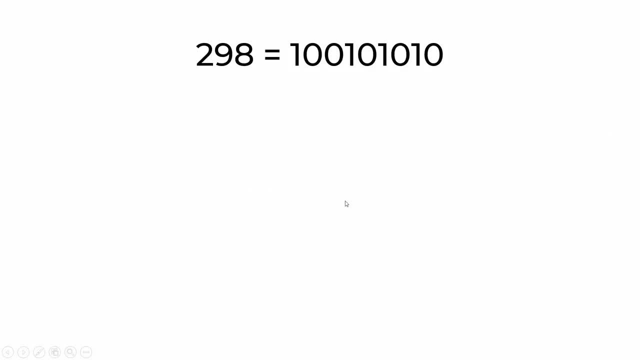 shown you. here is a simple diagram. In reality, we convert that number into binary number, So 298 is equal to this binary number. You can watch other videos on how to convert a number into binary, but there is some formula that you apply and you get binary number. So here each single digit is a bit, which. 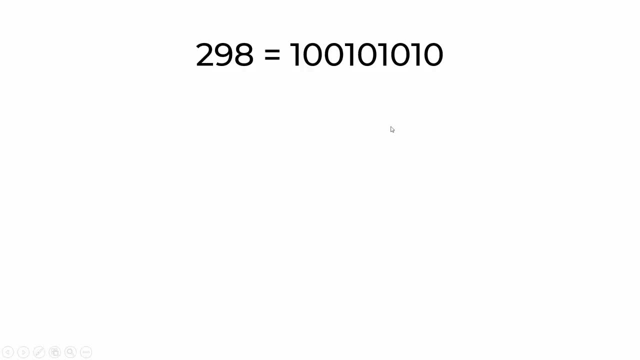 could be either 0 or 1, and when you have an integer number you use 4 bytes to store the number. 4 bytes is the capacity of integer number in many programming languages. Hence you store 298 like this. So one byte is 8 bits. So you can see. 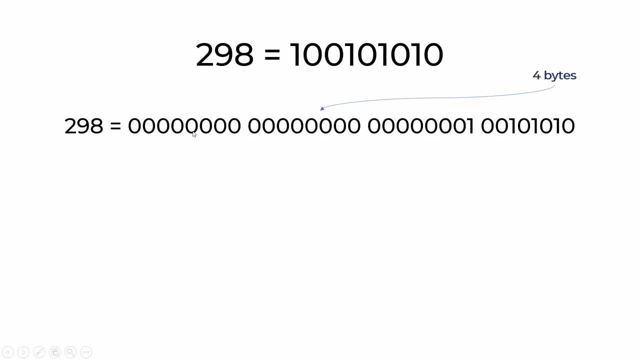 that this is 8, this is 8,, 8 and 8.. Now you have 4 bytes. These 4 bytes are actually stored on memory location, So 298 is stored like this. So in reality, the stock prices of apples are: 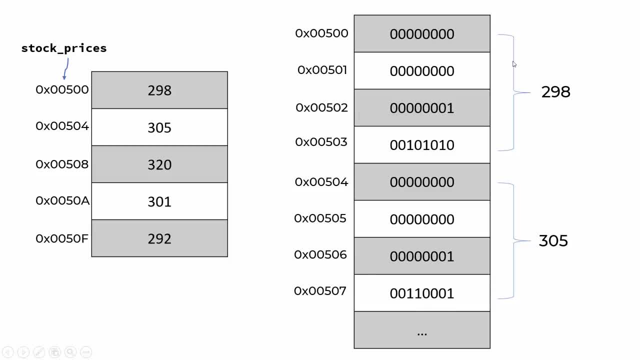 stored in a way that is shown on the right hand side diagram. And you know there are addresses like 500 is one byte, 501 is another byte, and so on. So 4 bytes for every number. But just to keep the presentation simple I'm gonna 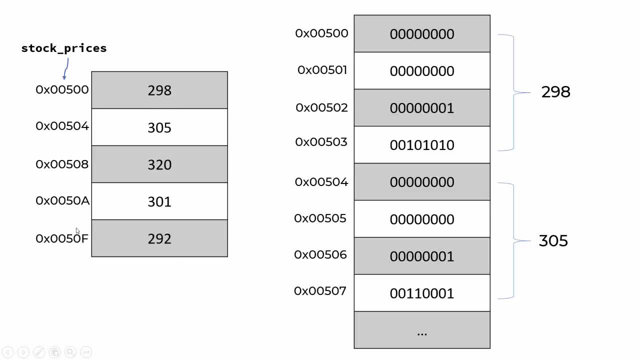 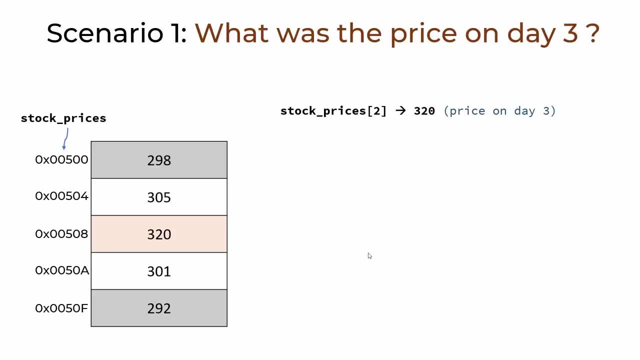 use the diagram on the left hand side. But just remember, internally it is all bits 1s and zeros. Now let's walk through some of the scenarios in our program. The first question you might ask your program was: what was the price on day 3?? For that you can use the index operator like this, Where you know the 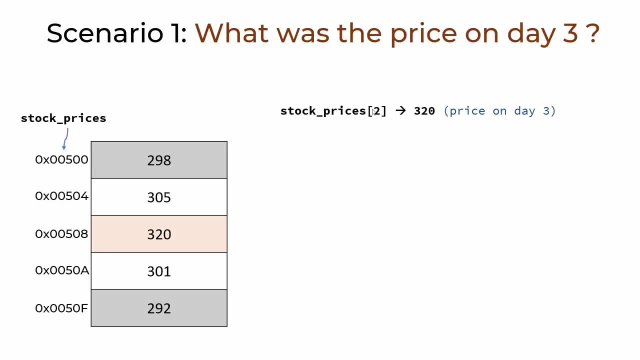 index starts from 0.. That's why the price on day 3 will be stock prices in index operator 2.. That will give you 320.. So let's see how it works under the hood. when stock prices is assigned this memory location, it is. 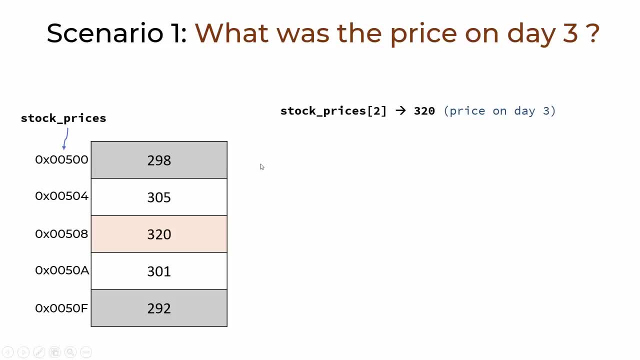 pointing to this particular memory address. okay, when you do index of 2, what it is doing is in that memory address. it will add 2 into size of integer because, see, size of integer is 4 byte, hence the first one is at 500 and, Oh, 504. okay, that. 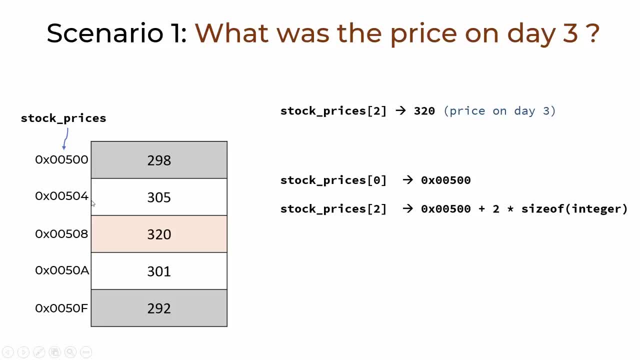 is your first. I mean, I'm starting from from 0th element, but in reality it's a second element. so second element is it is at 500, and fourth location, third element, is 508. hence you can use formula like this, which gives you an address: 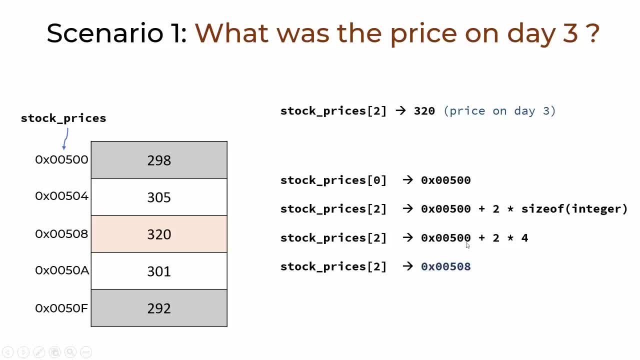 508. and if you have not watched this video, please do watch it from the link in the description. so now we are coming to our next step. and finally, it is our next step because, if you have not watched this video, please do watch it from the link in the description. so now we are coming to our next step, because if you have not watched, 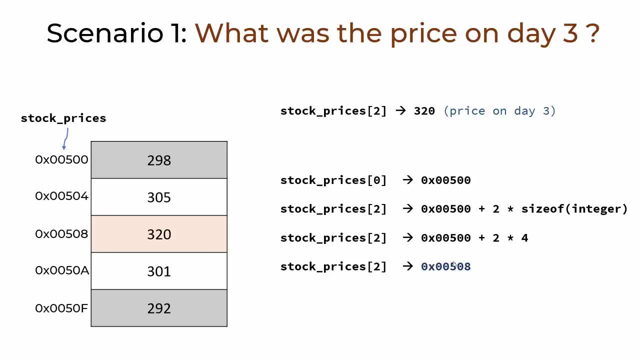 my big O notation tutorial. please watch it because throughout the data structure series we are going to evaluate big O complexity of our program, which tells you how much time your program is going to take in terms of big O notation. and this is a common question you get during any programming interview. so it's better. 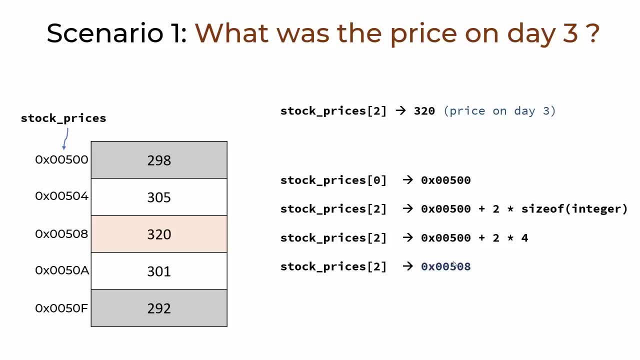 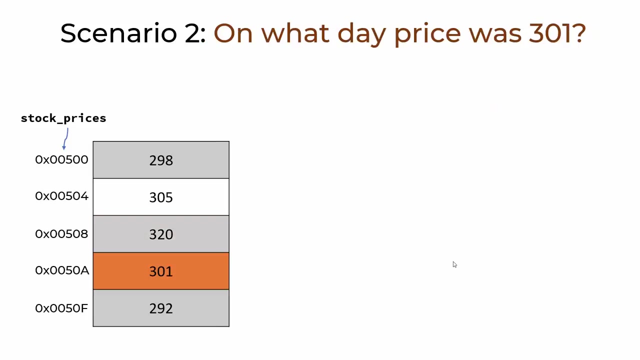 that you get your understanding clear on big O notation. so here the index lookup for an array will be order of one. so the big O complexity of looking at an array element by index is order of one. order of one means it is constant time operation. the second scenario is on what day? the price was 301. so here you are. 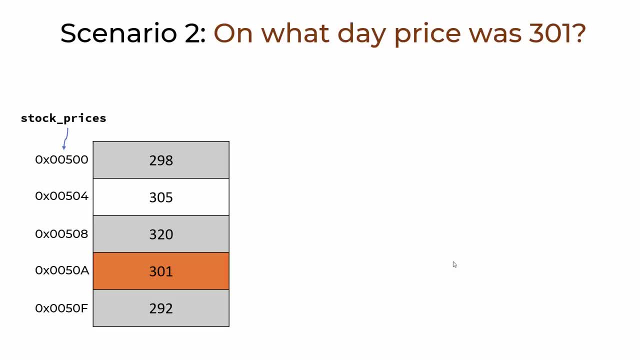 not going to be able to calculate the price of the array, but you are going to. not looking by index, you are looking by value. a simple Python program can be running a for loop on your values and comparing these values one by one. when you get 301, you return that value or print it. okay, you are doing n number of. 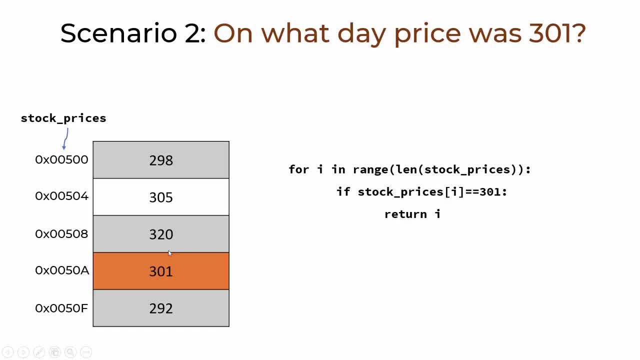 iteration in this loop. so let's say, if you're looking for 292 element, you have to go through all the elements in the list, and big O complexity is often looking at worst-case analysis. hence the complexity for this program will be order of n, which means you have to do n number of iteration to find the value in. 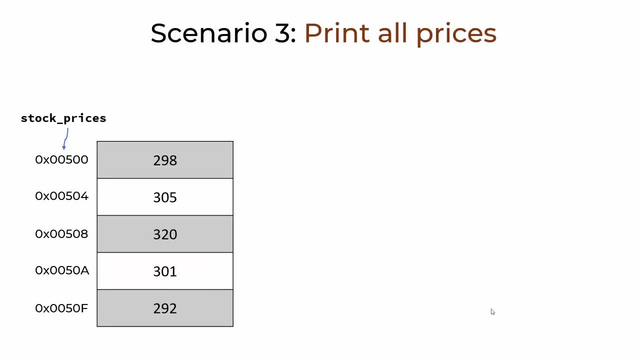 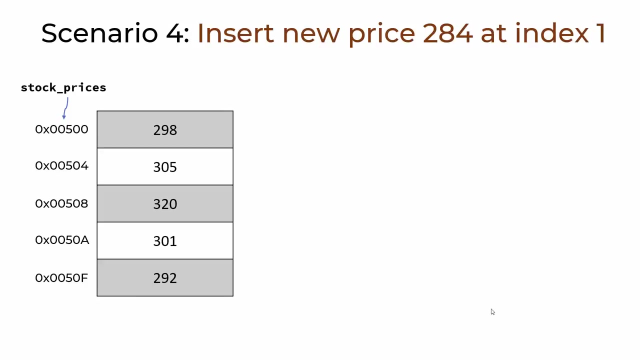 the array. third scenario is you want to print simply all the prices or you want to do a traversal. in that case you can just go through all the elements in the for loop and just print them. the complexity of this program is also. order of n. you want to now insert a prize at a given index. 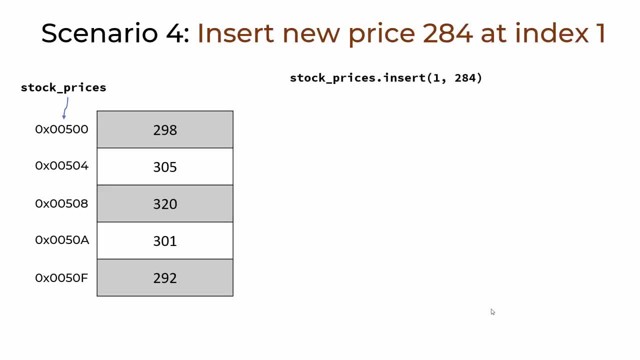 so what will you do? you will use insert function in python, which takes the index as a first argument. the second argument is the value that you want to insert. when you insert the value, after inserting the value at the first location, it will shift all the elements by one position. 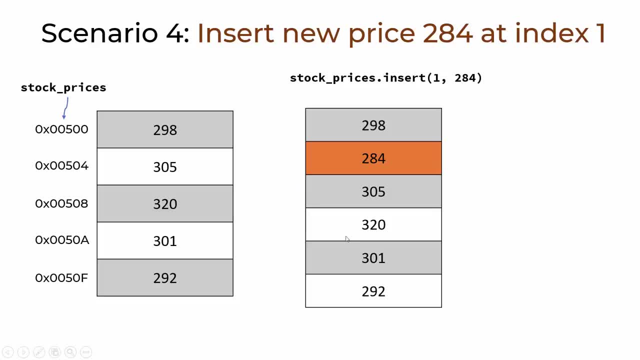 so say 305, it shifted to the next memory address. so since you are doing all these swaps, the complexity of this program is order of n because you have to do n number of swaps. deleting element is also similar. let's say you want to delete 305, the function that you use in. 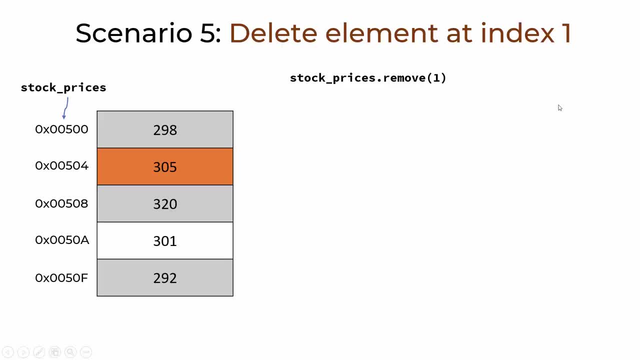 python is dot remove, you supply index as an argument. so 305 is 1 at 1 index. after it removes the element, it has to uh, shift this elements upwards, so 320, it will move up and so on. so again, the complexity of this program is order of n. now in python the actual memory presentation is little different, because python 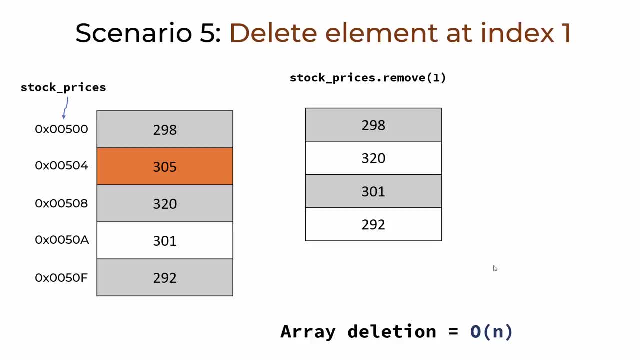 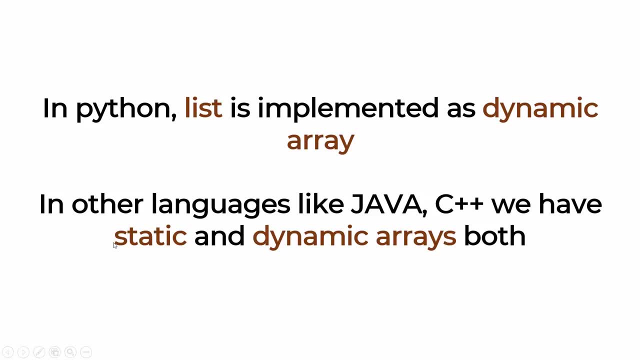 uses objects and references, but i'm just giving you a simple presentation so that you understand the concept behind an array. okay, in python, the list that we used is actually a dynamic array. arrays are of two type: static arrays and dynamic arrays. in java and c plus plus, they have both. 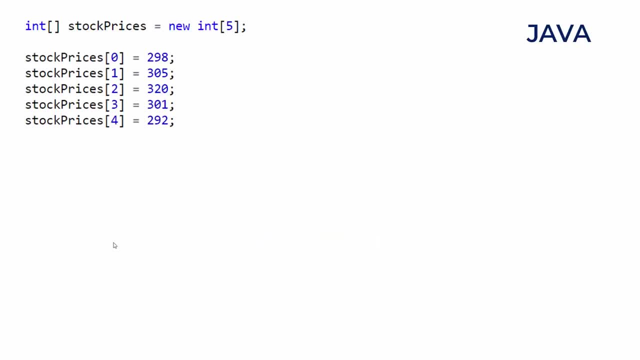 static and dynamic arrays. so let's say you're writing a program in java to store the same stock prices. one way you can do it is by creating an integer- integer array of fixed size. when you do new int file it will create an array of fixed size, which is five here. so when you try to insert an 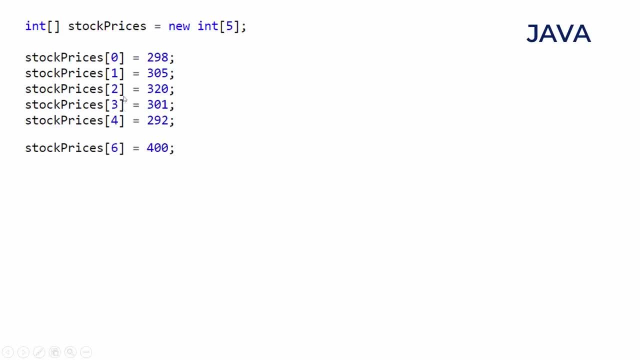 element. at this point, it will create an array of fixed size, which is five here. so when you try to insert an element at the seventh position- okay, since it is starting from zero, six will be a seventh position. this will give you an exception. your program will crash. it will not allow it because this: 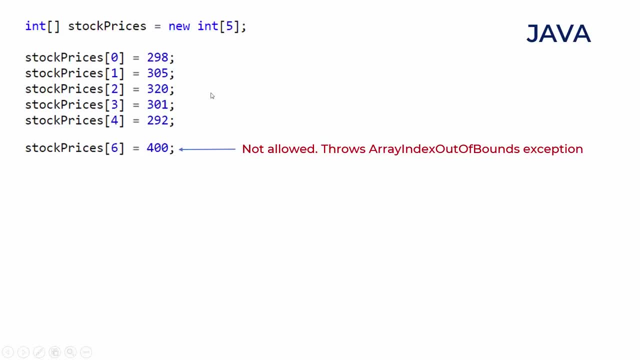 is a static array. in static array, when the size is fixed, you cannot insert elements beyond your size. the other type is dynamic array, or a list. in java is an example of dynamic array. you don't have to specify any size here. you can keep on adding elements and it just dynamically grows. the first 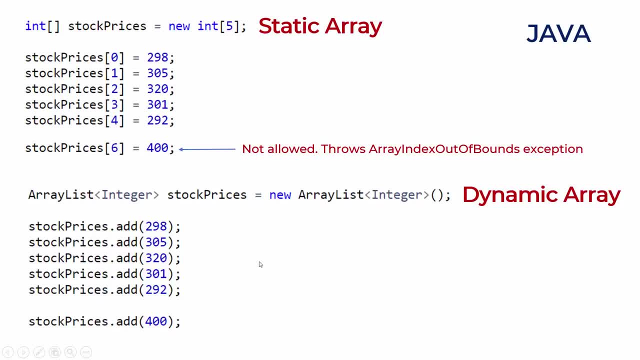 one was static array. the second one is dynamic array. now let's look at how these static and dynamic array work under the hood. static array is very simple. you have fixed size and it will only allocate the memory for that fixed size. okay. but for dynamic array, when you create your array object, 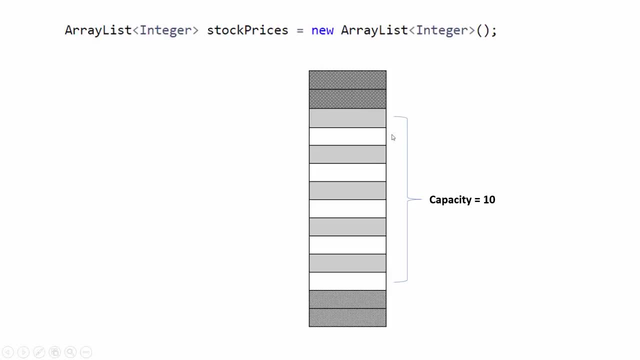 like this: it will allocate some integer variables for it. but when you create an array in static array you just need to create a fixed size because you want it to be static, and if you add some of that Initial capacity in the memory, Okay. So let's say all these boxes, the stand boxes. 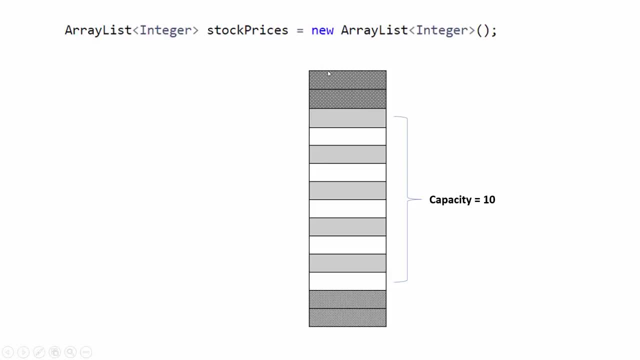 it allocated it for the stock prices array and The gray boxes I have shown at the top and bottom is, let's say, this is a continuous memory area and these Locations might be used by some other program, or maybe might it might be used by other Variables in the same program. So these gray boxes are not available for use to you. 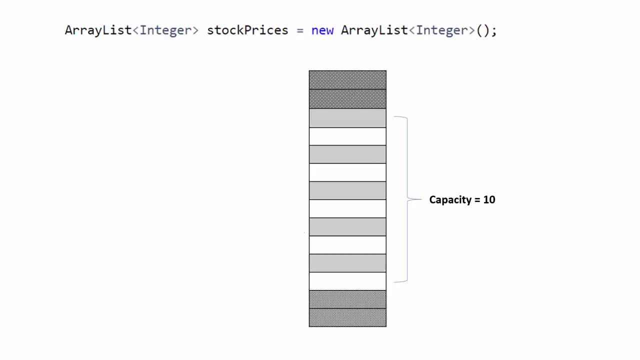 When you created this array, it created initial capacity of 10 and it will see if that capacity is enough. So what happens is, when you insert these elements, it will keep on inserting. Okay, so it will insert this six elements. fine, What happens after you insert 10 elements? So let's check that. So let's say you inserted 10 elements, your capacity is over. 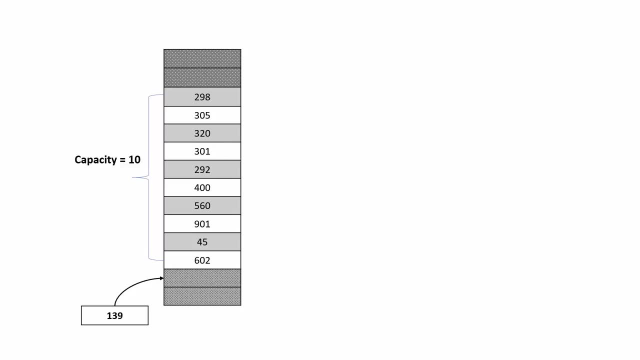 Now you want to insert 139. in that case, what it will do is it will allocate One new memory area at a different location. So let's say, at a different location It will allocate a total Capacity of 30. so 10 was the initial capacity and the new capacity it is going to insert will be current capacity. 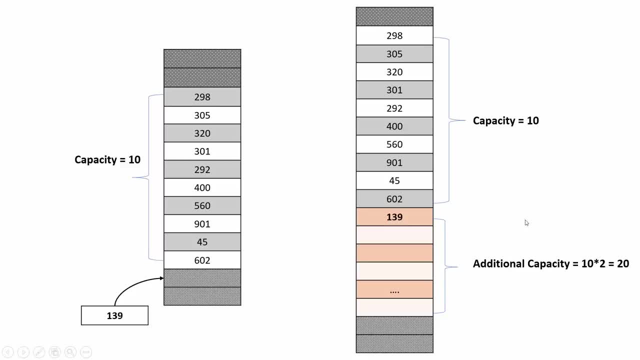 Which is 10? Multiplied by 2, so it will give you additional 20 spaces. So 10 spaces you already have. now you will have total 30 spaces, and then it will copy all These elements to new area. So you see, you have to do this copy and then it will insert. 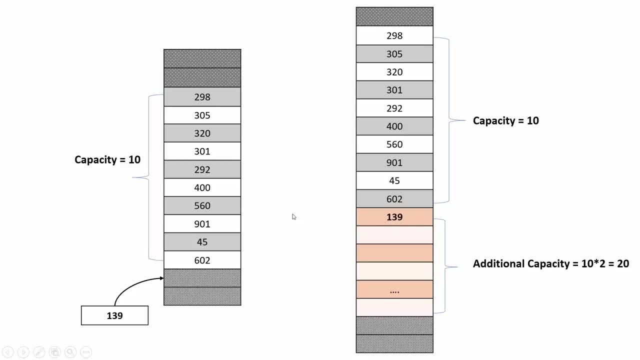 139, when arrays- dynamic arrays- grow, there is an overhead of allocating new memory and Copying all the elements. So now let's say you are at 30 capacity. if a 30 capacity is over when you try to Insert 30 first element, it will again allocate new memory segment somewhere else in the memory area. and 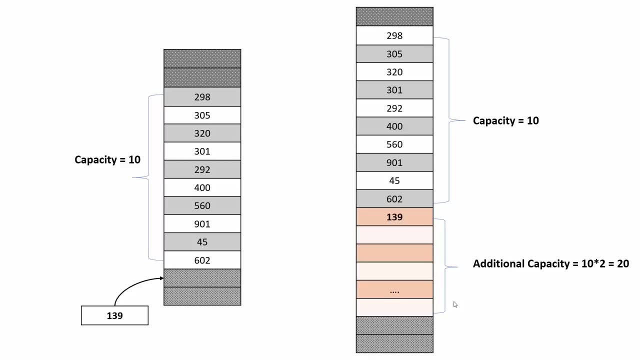 It will now allocate 30, which is a current capacity, and then 30 multiplied by 2, which is 60, So now your new capacity will be 90.. This is called geometric progression, if you know about mathematical geometric progression. so that's how these arrays work, so that they can handle the load of new insertion and insertion. 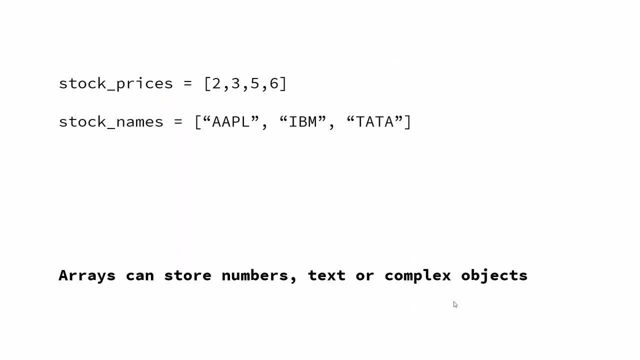 arrays can store Numbers. they can store tags like this. They can even store a complex objects. The thing about Python is Python can even store multiple types of element. Python can store integer and text both in the same array, but Java and C++ cannot do it there. The type is fixed.